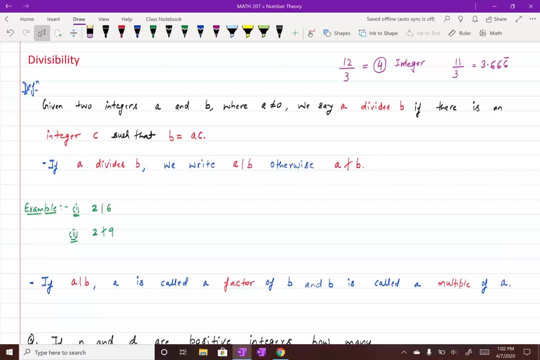 So you learn one important thing here: that when you divide 12 by 3, you will produce an integer 4, but when you divide 11 by 3, you will get the value 3.666 is not going to be an integer, okay, so say not integer. 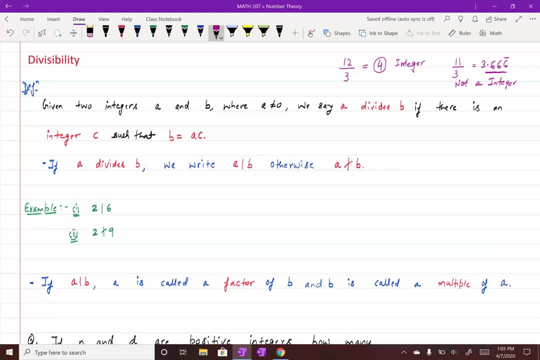 So if you want to classify, when can you say if you divide a integer by a non-zero integer? Say, if you divide a integer by a non-zero integer and you will produce integer, and when it's going to happen that you're going to divide integer with a non-zero integer and you're not going to produce. 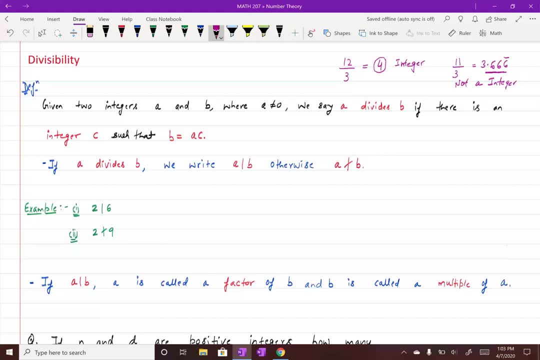 integer. okay, so divisibility is the concept which you're going to use when you divide an integer with a non-zero integer, and you will produce an integer, so it will classify your first case. okay, so the concept which we can define based on this definition. so, given two integers, a and B, where a is not equal to zero, we: 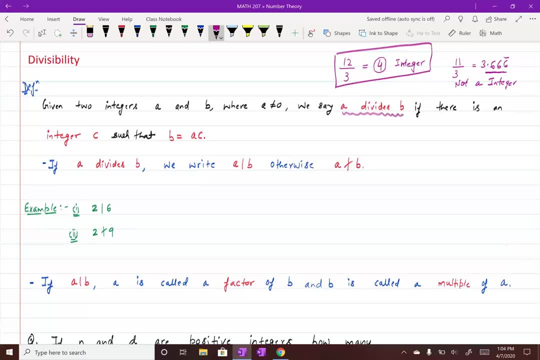 say a divides B, if there exists another integer, C, such that B can be represented as a times one of C. so here you are saying you can say a divides B. so if you have a P and you divide that by a, where a is a non-zero integer, then if you can produce another, 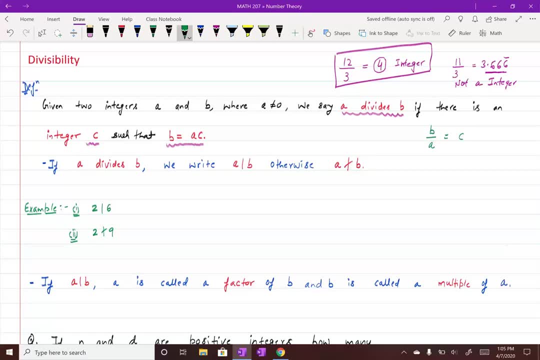 integer C: okay. so if that happened, then your statement that a divides B is going to be a true statement. okay. and in another way you can say: if you can represent B as some C times of a, we are C as some C times of a, we are C as some C times of a, we are C as some C times of a. 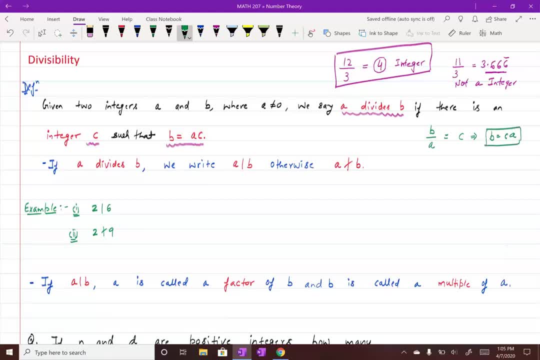 and they are your integers. there is another way you can say: a divides B. here we are going to follow this notation that if a divides B, so we can write with this notation that a divides B. otherwise, if a does not divide B, we can follow this notation that a does not divide B. so in our first example we're going to: 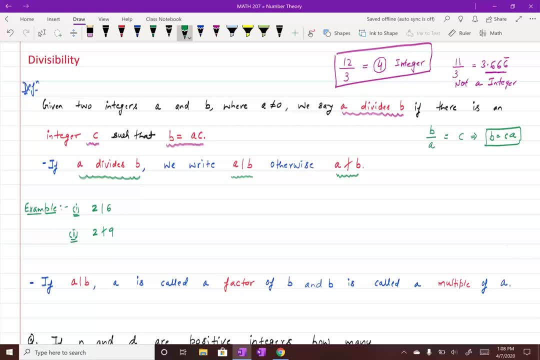 read as 2 divided 6, which is a true statement, because 6 can be written as 2 times of 3, there exists an integer 3 and 6 can be represented as 2 times of 3, while in the second example you are saying 2 does not. 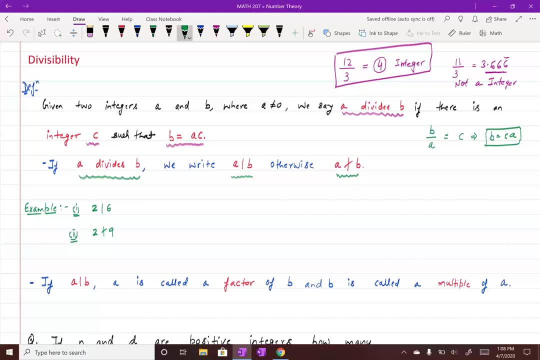 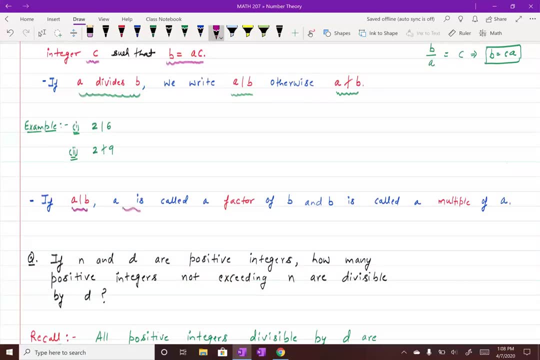 divide 9, because you cannot find another integer such that 9 can be written as 2 times of that integer. if a divides B, then a is called a factor of B and B is called here a multiple of a. okay, that's the relationship they have with each other. so whenever you have a 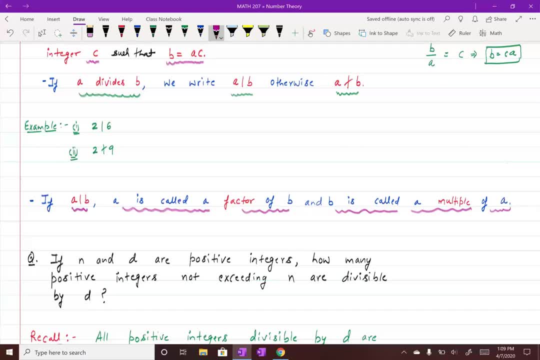 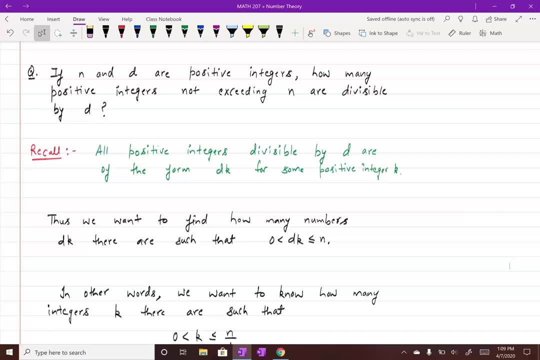 divides B. a is called a factor of B and B is called a multiple of a. so, based on this concept of divisibility, you can ask this question that if n and D are positive integers, then how many positive integers not exceeding n are divisible by this factor D? 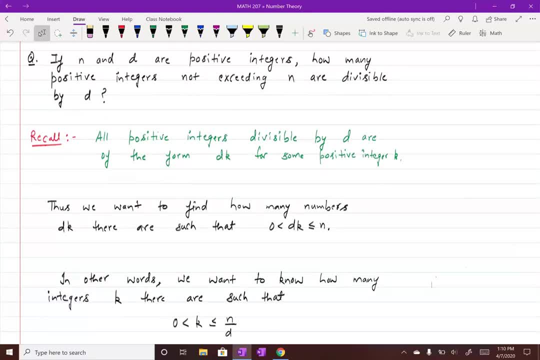 now from the concept of a divisibility, you can say: all positive integers and divisible by D are going to be of the form of a D times of K. so all positive integers which are divisible by D, you can represent them in the form of this M, where M is written as D, times of K, where K is some positive integer. thus, 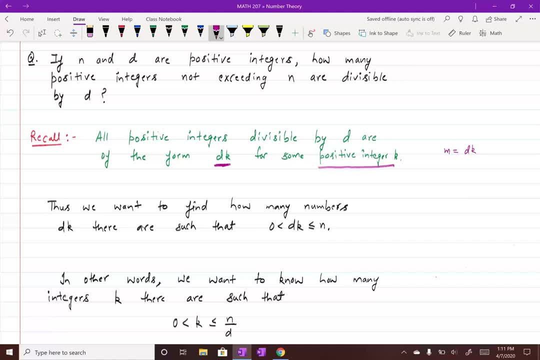 we want to find out how many numbers are this? d times of k are there such that they are greater than 0 and they are not going to exceed than n? because that's the question you are asking here, that how many positive integers not exceeding n are divisible by d. So, since they are the positive integer, 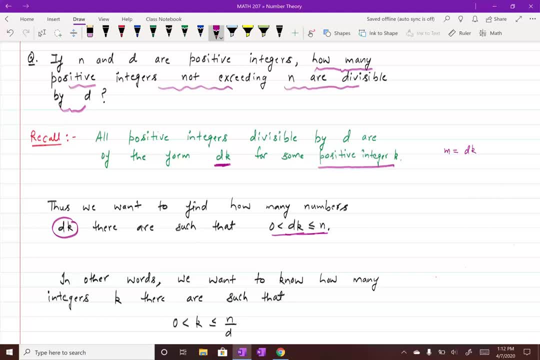 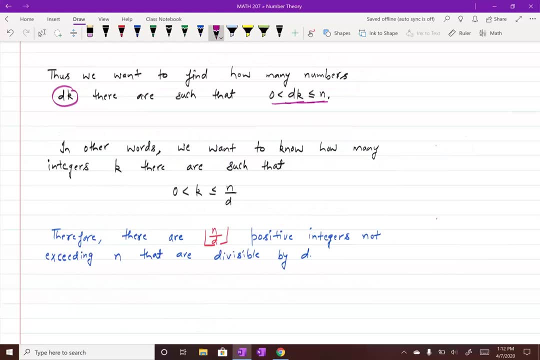 this d times of k is greater than 0 and they are not exceeding than n, so it's going to be less than equal to n If you divide this inequality by your factor d. so you can say in another words: we want to know how many integers k are there such that my k is greater. 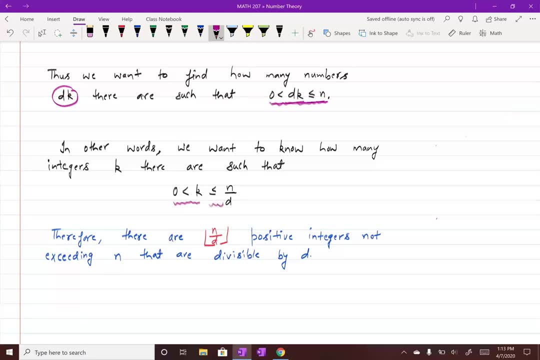 than 0 and less than equal to n divided by d. Okay, and you can find those number of integers, k, By following your floor definition. so there are the floor value of n divided by d, positive integers not exceeding n that are divisible by your factor d. Okay, so that's going to. 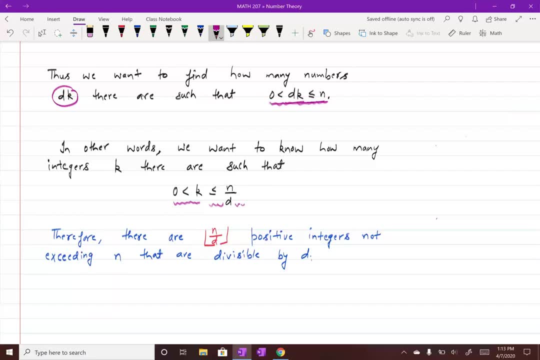 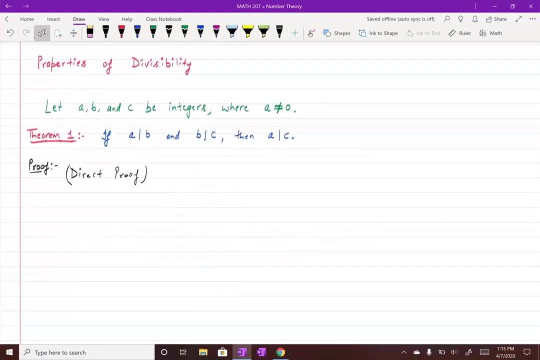 be the solution of your problem and you are able to know all those positive integers just by applying the concept of divisibility there. Okay, So you can say those number of integers- positive integers, are going to be the floor value of n divided by d. 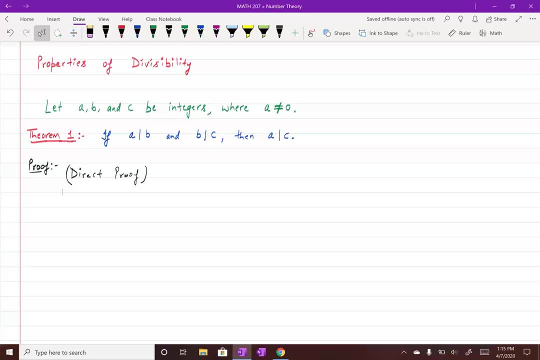 So, based on this concept of divisibility, we can prove our first result. So let a, b and c are integers and a is not going to be equal to 0. Then your first statement is: if a divides b and if b is not going to be equal to 0, then your first statement is: if a divides b and 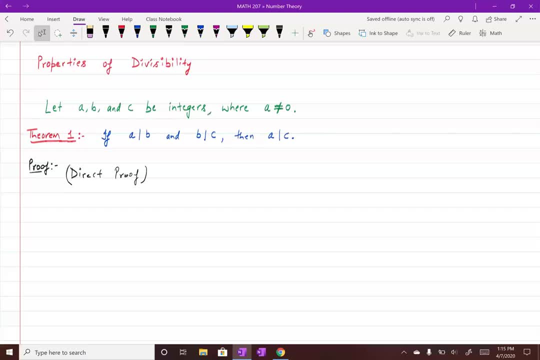 if b divides c, then can you conclude that a also divides c. Okay, As in writing the proof of this statement, we can follow our diet proof technical. So in a diet proof technique you start by assuming, Let's suppose, your hypothesis, which is a, a. 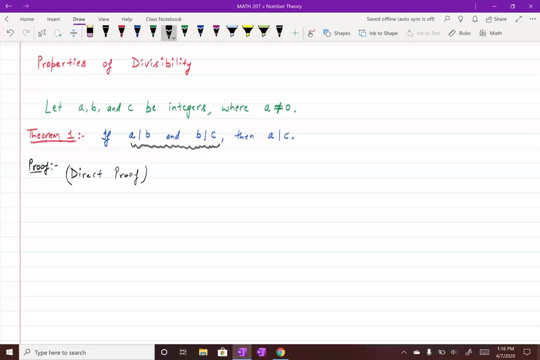 divided b and b divided c here. Let's suppose that hypothesis true. Then under that hypothesis can you also prove that your conclusion is also accurate? Here your hypothesis is true. Can you confirm that your hypothesis is also correct? Here your hypothesis is correct To. 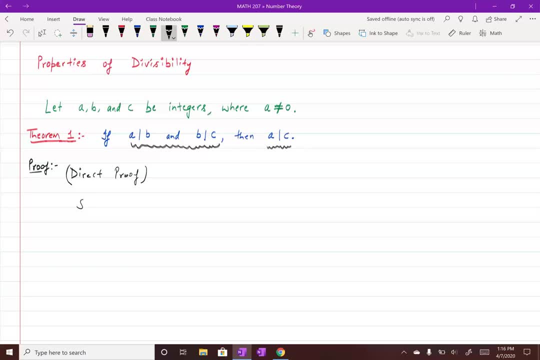 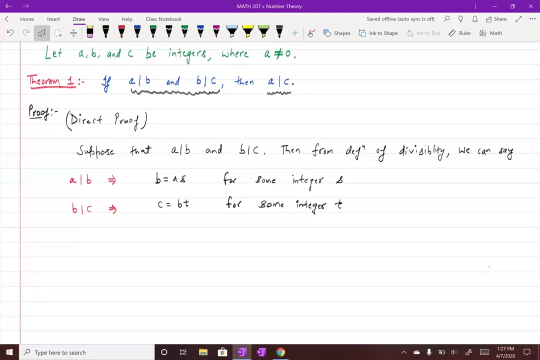 also going to be true, and your conclusion here is: A divides C. So suppose that A divides B and B divides C. okay, Then from the definition of a divisibility we can say: A divides B implies that B can be written as A times of S, for some integer S, and B divides C. that means 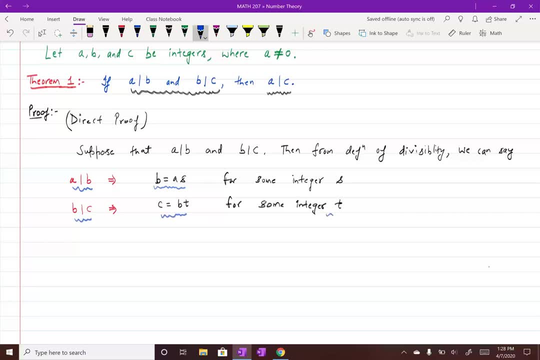 C can be written as B times of T for some integer T. Now if you take this as your first equation and this is your second equation, then on combining first and second, first and second, first and second, we get that C is going to be equal to B times of T, which you can write as A times of S times. 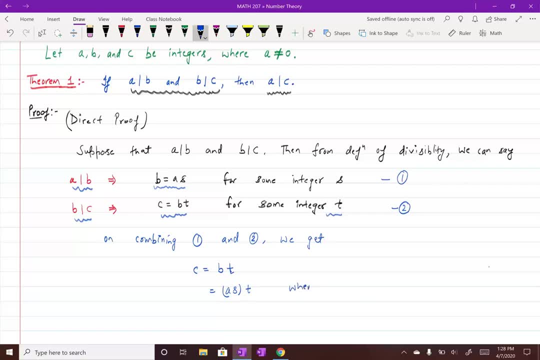 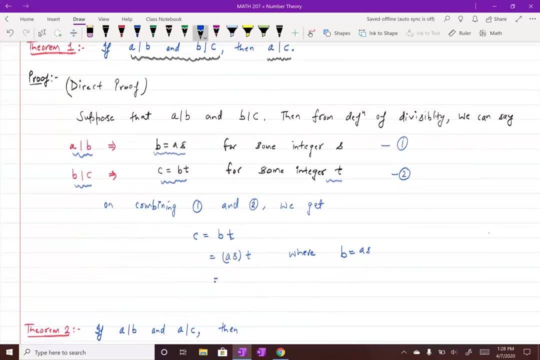 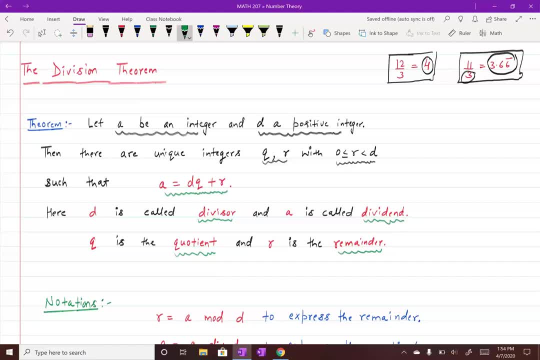 to be equal to A times of T, where you have used the fact that B is going to be equal to A times of T, where you have used the fact that B is going to be equal to A times of came cases based on your division theorem. So here, if a is 11 and d is your 3, so the 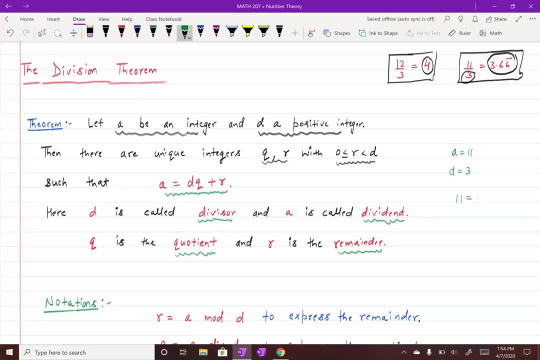 11 can be written as 3 times of 3 plus of 2, then your cosine Q here is 3 and your remainder r here is going to be equal to 2.. Remember, whenever you have the value of r equal to 0, you will again represent the concept of divisibility there. In that case a can be. 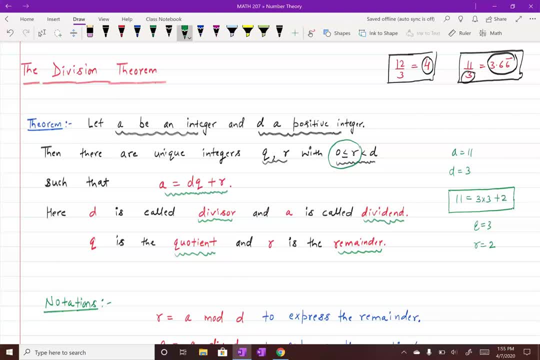 written as a multiple of d for some integer Q, but if the value of r is greater than 0 and less than d, then this is a representation of the case when you divide an integer by a positive integer and you will produce something other than integer. 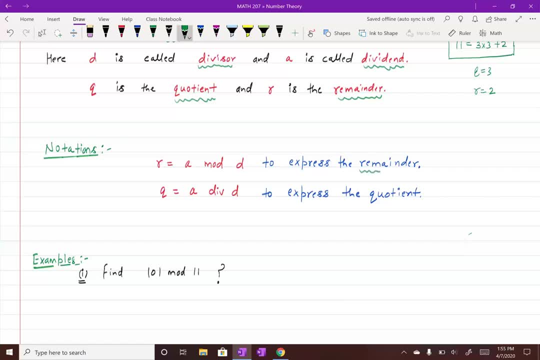 The common terminology to express your remainder term, r. the r based on your divide and a and divisor d. you can say r is basically equal to a mod d, which is the notation to express your remainder term. And the cosine Q can be expressed with the help of a divide and. 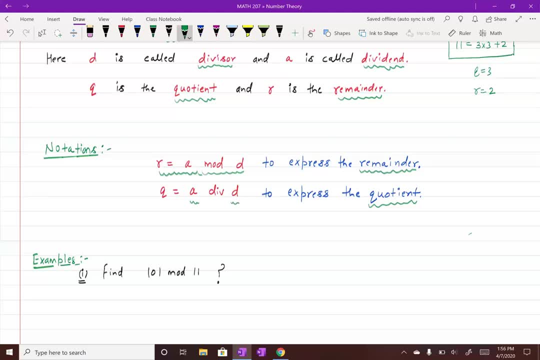 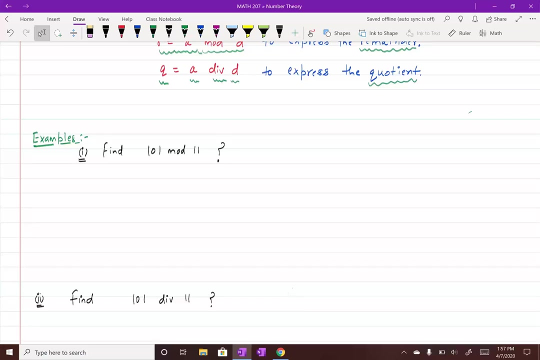 a, The notation which you are going to use to define your cosine. Q is a div and d. So Q can be represented as a div d and remainder r can be represented as a mod d. So if you have to find this cosine and remainder value in the case when you divide 101 by 11,, 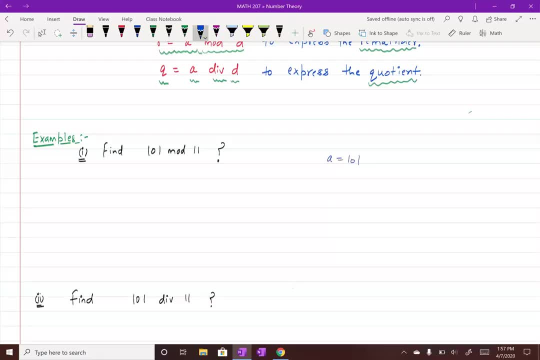 So your a in this case is 101 and your d in this case is 11.. Now, by following your division algorithm, you can say: 101 can be written as 11 times of 9 plus of 2.. And this gives you that your quotient in this case is 9 and your remainder in this case, is 2.. 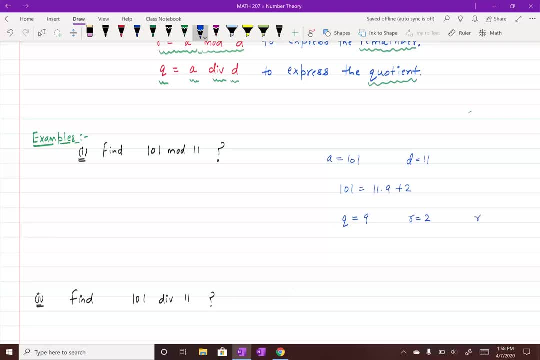 And your remainder is going to satisfy the definition that r is going to be greater than equal to 0 and less than d. That means r is going to be greater than equal to 0 and less than d- 11 here. and you have the value of r equal to 2 here And the value of cosine q is equal to 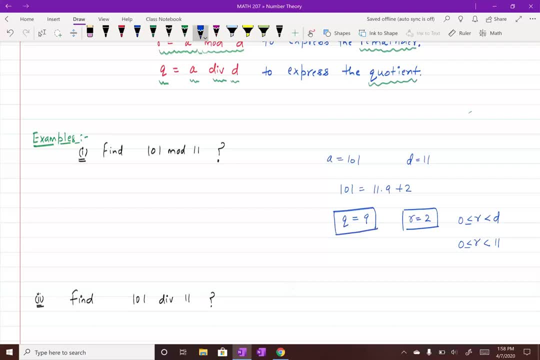 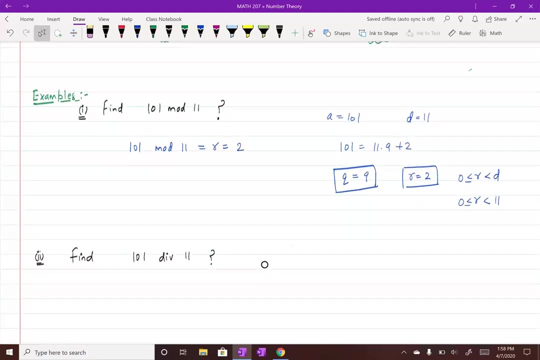 9 here. So, based on this notation, we can say: the 101 mode of 11 is basically your remainder r and your remainder r is going to be greater than or equal to 0.. So, based on this notation, we can say that your quotient in this case is equal to 2.. Similarly, you can get the value of 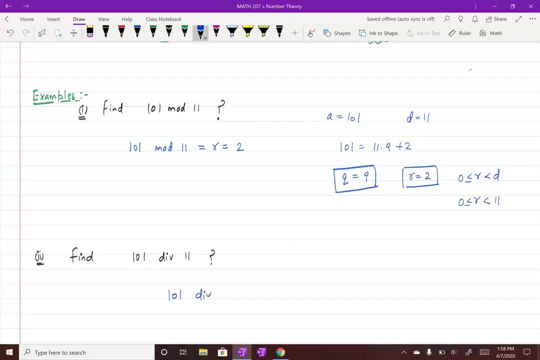 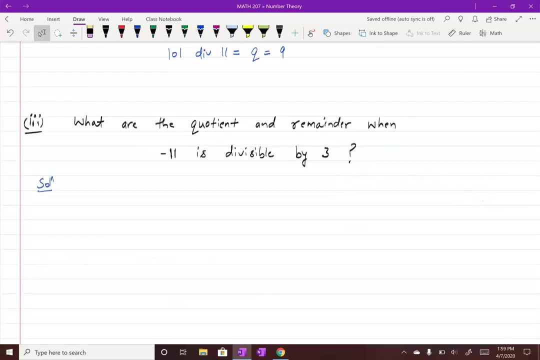 101 div 11, which is basically your quotient q, and the quotient q in this case is going to be equal to 9.. Now if we take another example, and this time you are supposed to find the quotient and remainder in the case when you have a dividend equal to minus 11 and is divisible by 3.. So 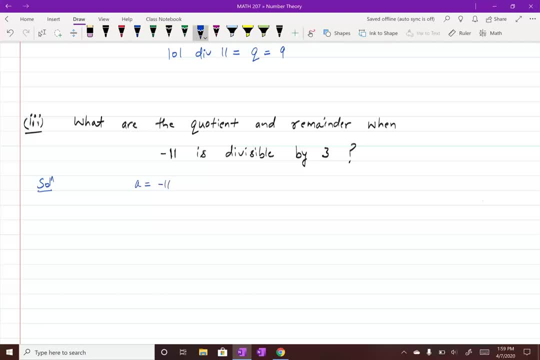 in this case, you can get the value of 101 div 11, which is basically your quotient q and the. In this case, your a is going to be equal to minus of 11,. your d is going to be equal to 3.. And based. 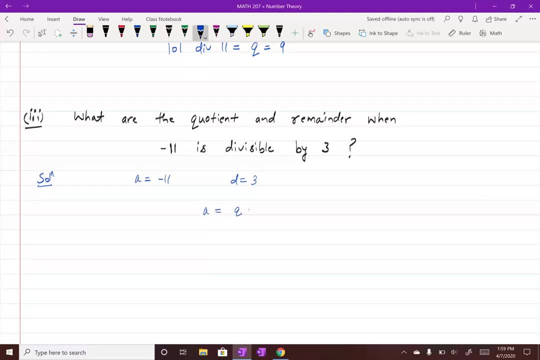 on your division algorithm. a can be written as q times of d plus of r, where r is going to be greater than equal to 0 and less than d. So minus of 11 can be written as 3 times of minus of 4, and. 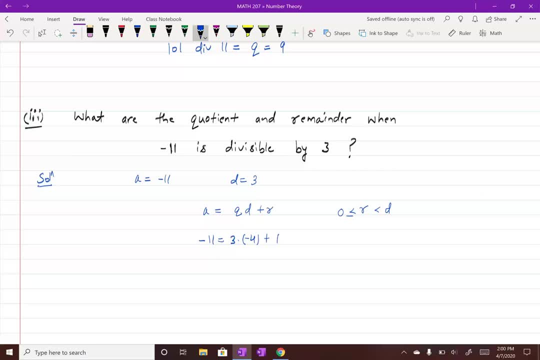 plus of 4.. So you can get the value of 101 div 11, which is basically your quotient q and the of 1.. So in that case your quotient q will be equal to minus of 4 and your remainder r will. 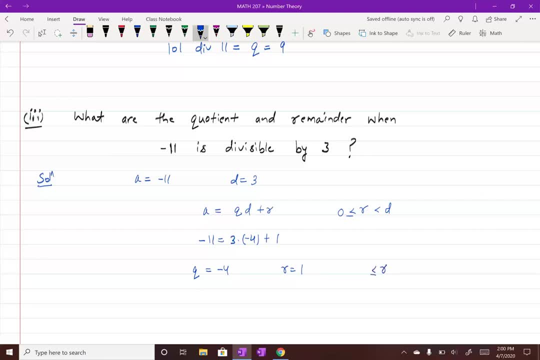 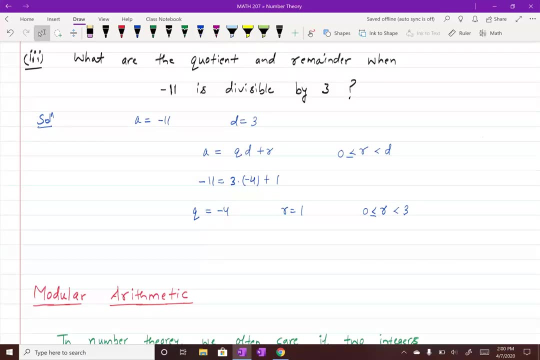 be equal to 1.. And this r is going to satisfy the condition. r is greater than or equal to 0 and less than. So remember you could have another case to represent your minus of 11.. You could have think that minus of 11 can also be written as 3 times of minus of 4,. 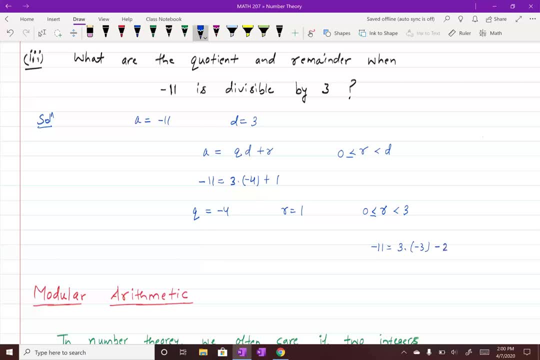 3 and then minus of 2, because this side 3 times of minus 3 is minus of 9, then minus of 2 is going to be equal to minus of 11. but this will not have hold the structure of your division algorithm because according to your division algorithm the A can be written as: 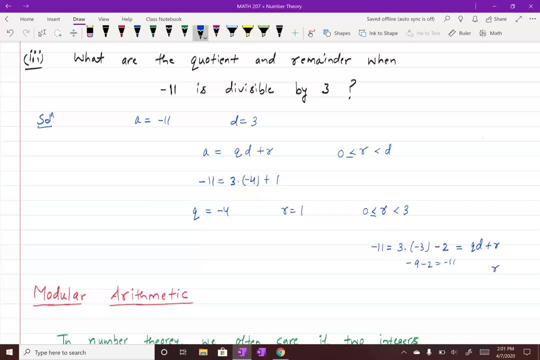 Q of D plus of R, but R has to be greater than equal to 0 and less than your D, which, in this case, R has to be greater than equal to 0 and less than your 3. and if you deciding to represent your minus of 11 as 3 times of minus of 3 and minus of 2, in that case the value of R you have chosen as: 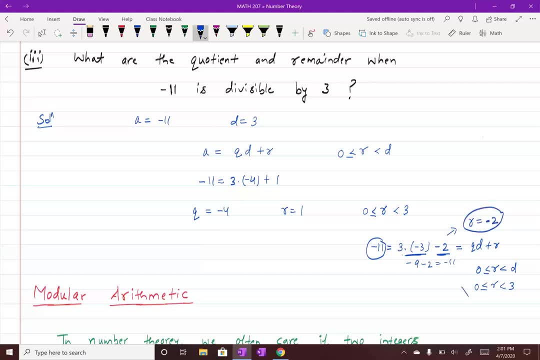 a minus of 2. and then you're going to contradict this condition that R has to be greater than equal to 0 and less than 3. okay, so you cannot consider this case to represent your integer minus of 11 when you divide by 3. 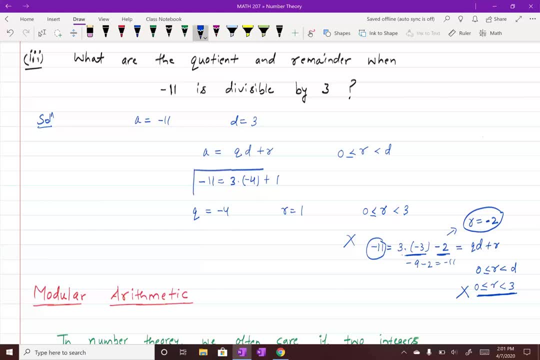 right. so you will only have this choice and, based on this choice, your quotient will be equal to minus 4 and your remainder equal to minus of 1. the another way you can represent this quotient, Q, as is going to be the floor value of A divided by D, so the floor value. 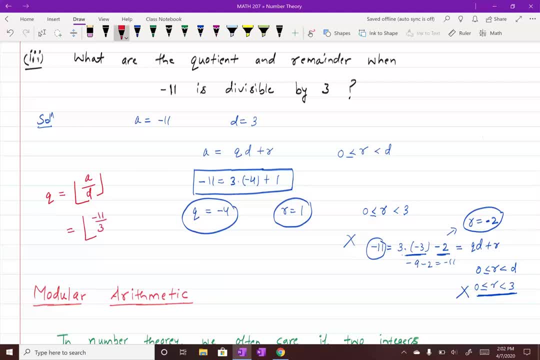 of A divided by D. here is minus of 11 divided by 3, as going to be the minus of 11 divided by 1, alright, of 4. once you get the value of your cosine, Q, then the remainder can be obtained as a minus D times of Q, which give you the value that R is going to be. 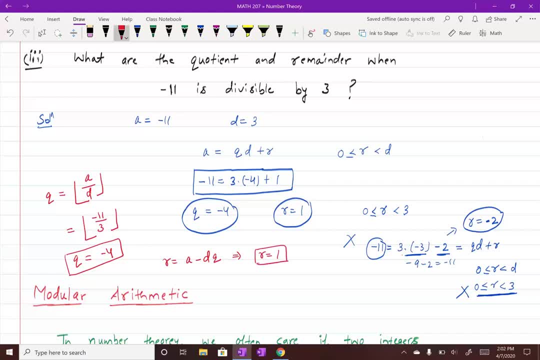 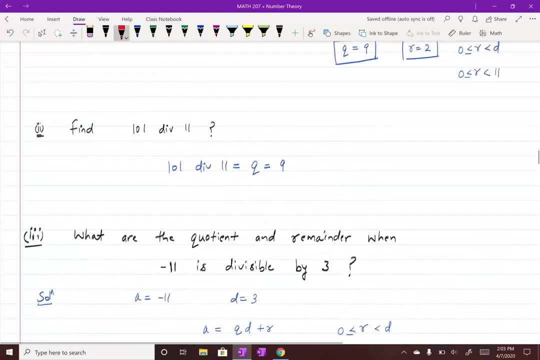 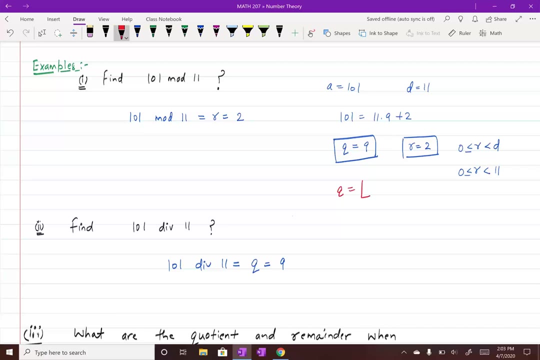 equal to 1 here. okay, that's another way you can compute your cosine based on your dividend and divisor. you can apply this result here. in the case of your earlier problem, the cosine Q was the floor value of a divided by D and a. in this case is 101 divided by 11. you will have 9 point something. so 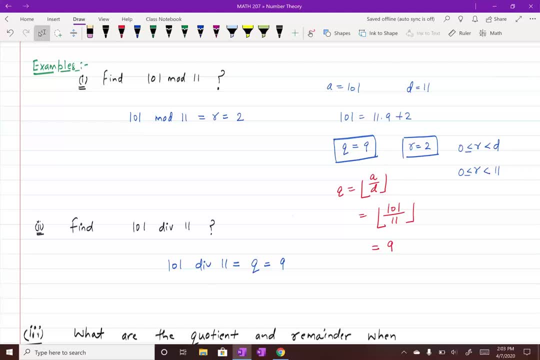 my cosine here is going to be equal to 9, and that gives you the value of remainder R based on the formula a minus D over Q, and a here is a 101. D is your 11 times Q is your 9, which gives you the value of R equal to 2. okay, 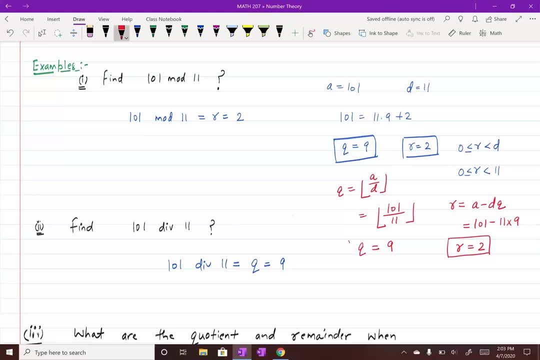 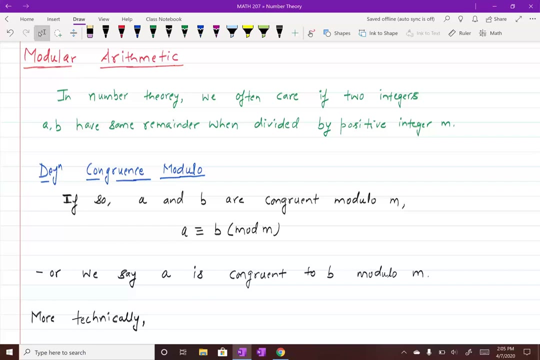 so there's another way you can compute the value of your cosine and your remainder by following this formula that the cosine can be computed based on the floor value of a divided by D in number theory, once we know how to compute the cosine and remainder, once you divide a dividend by a divisor. 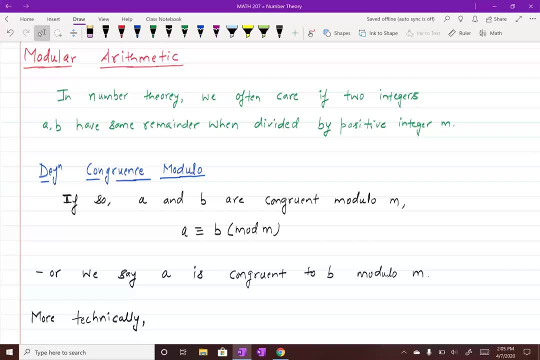 the next thing. we are interested in it in determining if you take two integers a and B and if you divide them with the same positive integer M, whether they will have the same remainder or not. and this gives you the definition of your congruence modulo. so, whenever you have two integers a and B and if they 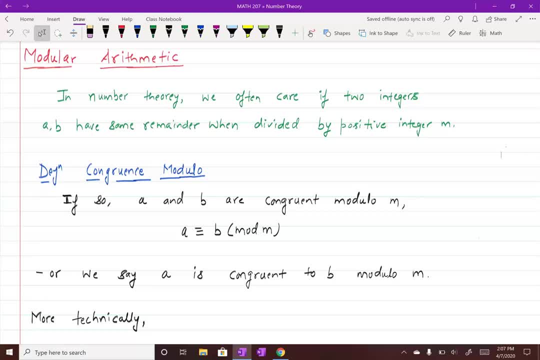 produce the same remainder when you divide them by a positive integer M, so you can say the integer a and B, they are related with the help of this relation which you can define based on your congruence modulo. so two integers, a and B, are related with the relation of a congruent modulo M, and you can write: 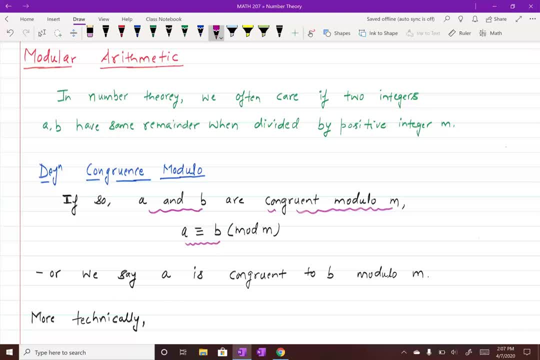 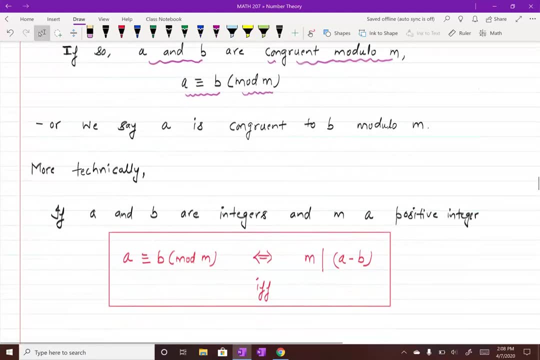 that a is congruent to be with modulus M. that means that if a and B are integers and M is a positive integer, then a is congruent to b modulo m if, and only if, m divides the difference of a minus b. ok, So, based on this concept, 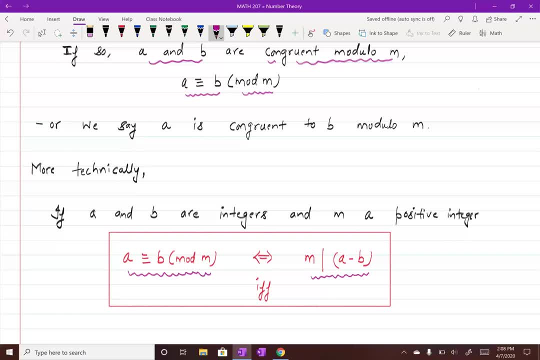 of divisibility you can find whether the integer a and b are related. and they can relate with this relation. we are going to say a is congruent to b modulo m. that means if we divide the integer a and b by positive integer m, they will produce the same remainder. and in another 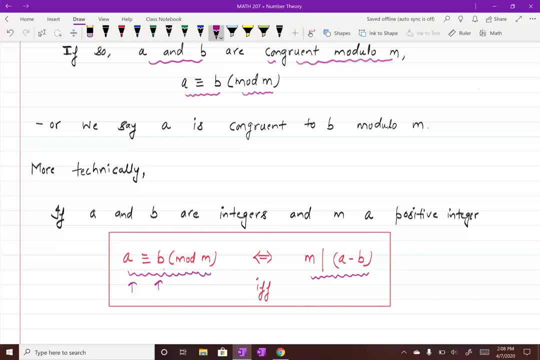 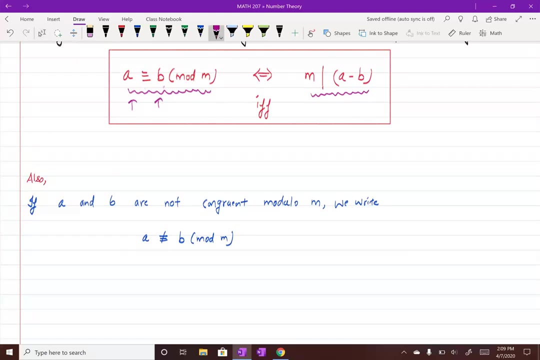 way you can say: the positive integer m divides a minus of b, because in that case the remainder will be zero. also, if a and b are not related with this congruent modulo m relation, then we are going to use this notation. we are going to say a is not congruent. 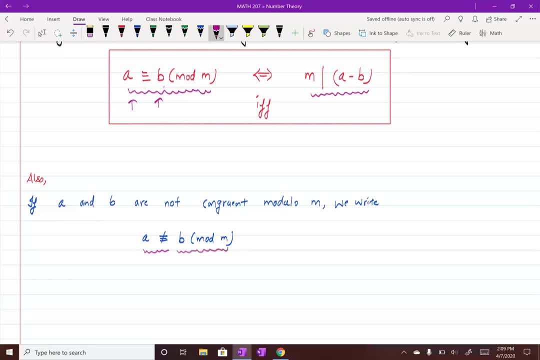 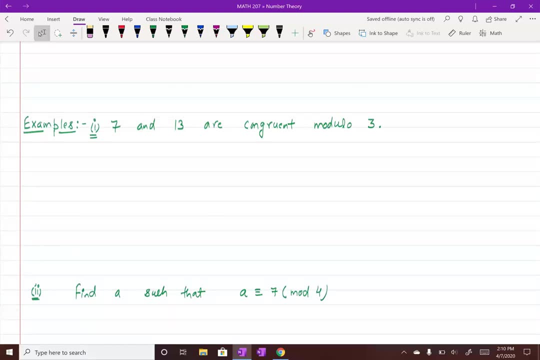 to b, B with modulo m. Let's take one example. So in our first example we are going to determine whether 7 and 13 are congruent- modulo 3.. So in that case we want to determine whether 7 can be written as congruent to 13 with a modulo of 3, okay, So if you look, 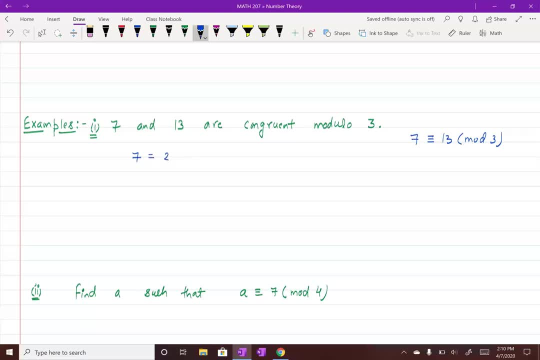 at 7,, 7 you can represent as 2 times of 3 plus of 1, okay. And if you look at the number, 13 can be represented as 4 times of 3 plus of 1.. So from here you get the cosine equal. 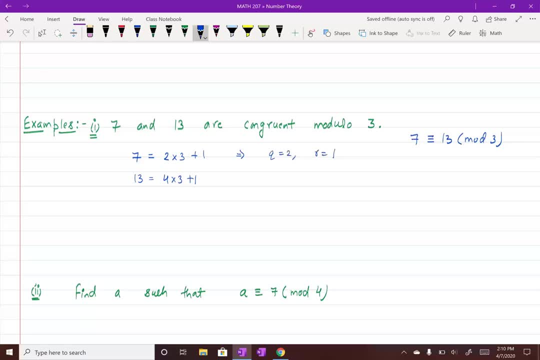 to 2 and remainder equal to 1, and from this relation you will get the cosine equal to 4.. and the remainder equal to 1. ok, So you can say that 3 divides 7 produce the remainder equal to 1, and 3 divides 13 also produce a remainder equal to 1.. And since the remainder 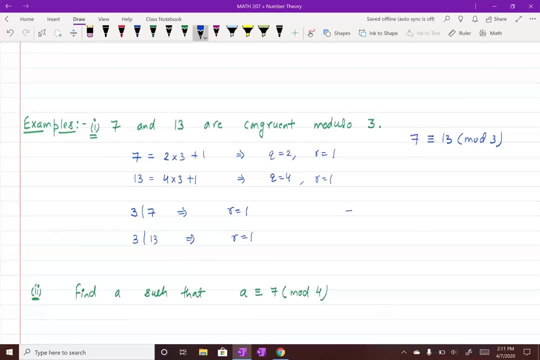 in both the cases are same, so you can have a relation between 7 and 13. and 7 is congruent to 13 with a model of 3. ok, The another way you could have a determine whether 7 is congruent to 13 with a model of 3, if we just take a difference between 13 minus of 7.. So 13 minus. 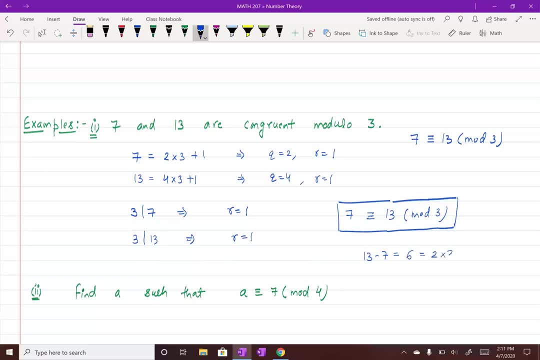 of 7 is 6, 6. you can write as 2 times of 3 plus of 0, the remainder is 0 in this case. So you can make any statement here that 3 divides your 13 minus of 7.. So you can write: 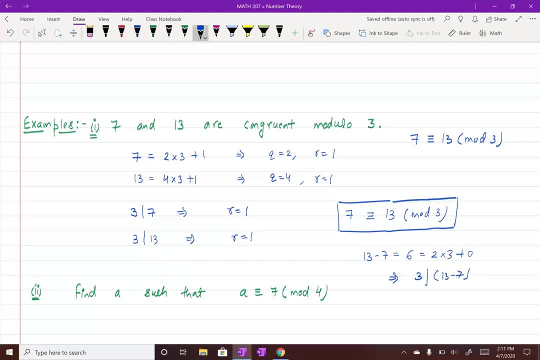 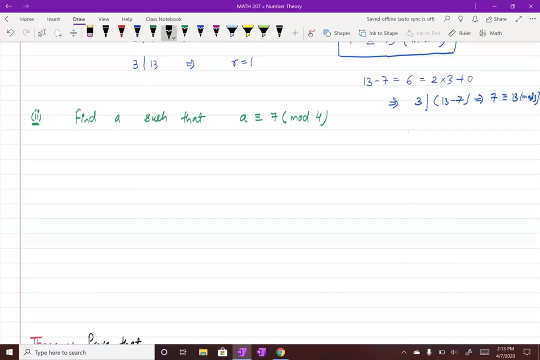 13 minus of 7 and since 3 divides 13 minus 7, so from your definition you can say that 7 is congruent to 13 with a model of 3. ok, Now in the second problem, you want to find an integer a such that a is related with 7. with this relation, that a can be written as: 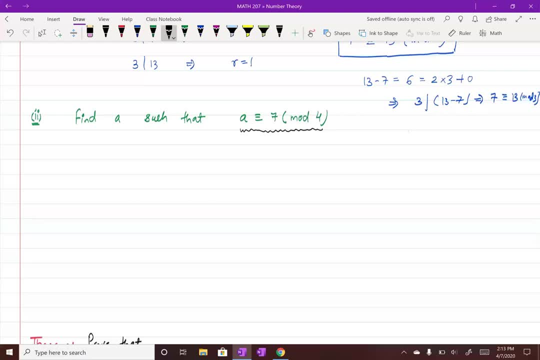 a is equal to 7.. So a is related with 7. with this relation that a can be written as a is congruent to 7 with a model of 4.. So either you can use this theorem that a is congruent. 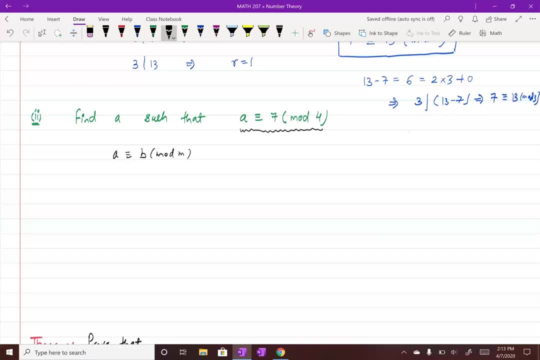 to b model of m, if, and only if, m divides your b minus of a: ok, So from here you can say: a is congruent to 7 with a model of 4 if, and only if, m divides your b minus of a. ok, So 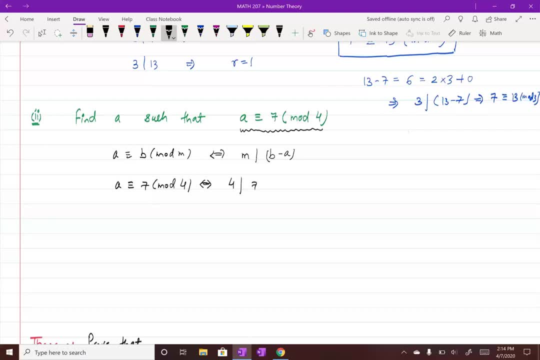 either you can use this theorem that a is related with b, with this relation, that a is congruent to 7, with a model of 4, if, and only if, m divides your b minus of a. ok, So either you can use this theorem that a is related with b plus of a, as such, that a can be written. 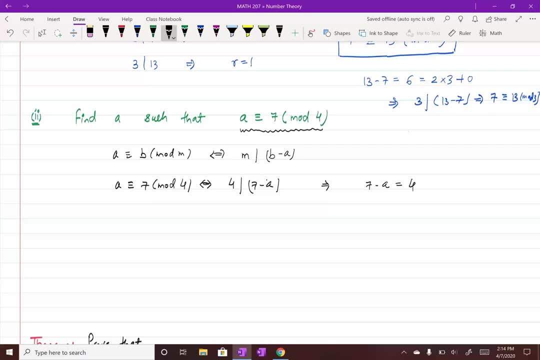 as b plus of a. ok, So whether you can do this and say that a is only if 4 divided by 7 minus of a, and if you apply the definition of divisibility, this implies that 7 minus of a can be written as 4 of some integer a. ok, and this implies a can be written as 4. 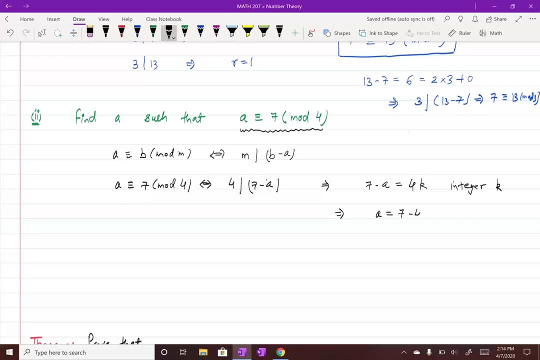 of some integer, a. ok, So this can be written as 26,, 26,, 28,, 28,, 29,, 33 or however many other. a can be written as 7 minus 4 of k. so your solution of this problem, a, could be of the form as 7 minus 4 of k for any integer. 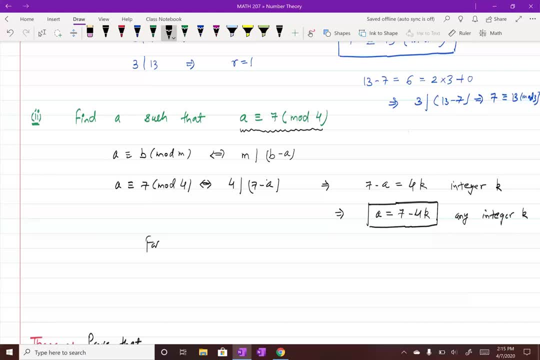 okay. so, for an example, the one value of a you can obtain by putting k equal to 1: if you put k equal to 1, then a is going to be equal to 7 minus 4 times of 1, which will be equal to 3. okay, and then you can easily check whether 3 is congruent to 7. 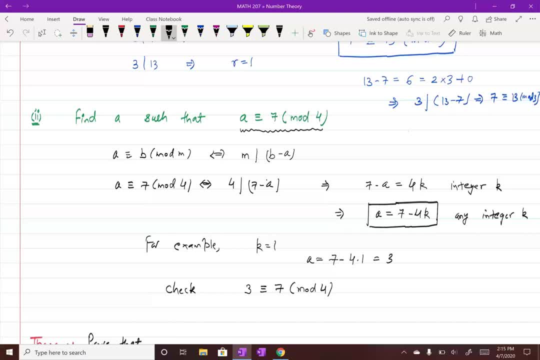 in mod 4, okay, and you can say from here: since 7 minus 3, okay, 7 minus 3 is 4 and 4 is a divisible by by 4. so this value of a will work here. so a could be equal to 3 and you could have put: 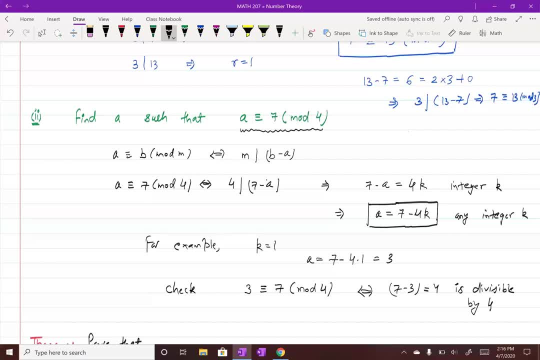 a more value of this integer k and you can produce the other values of your unknown a. okay, then other way you can check. 3 can be represent as 0 times of 4 plus of 3, so the remainder in this case is r equal to 3. if you look at your 7. 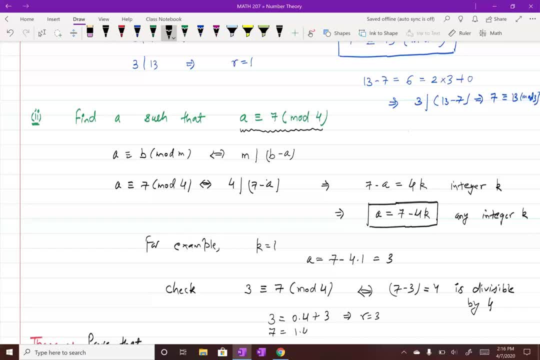 7 can also be written as 1 times of 4 plus of 3, so remainder in this case is also 3. so the 3 and 7, they are related with respect to this relation. that 3 is congruent to 7 with the. 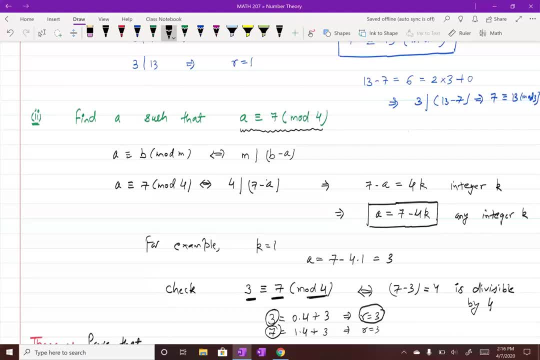 model of 4 because in both cases they produce the same number of values. so the 3 and 7: they are related with respect to this relation, that 3 is congruent to 7 with the model of 4 because in both cases they produce the same number of values. 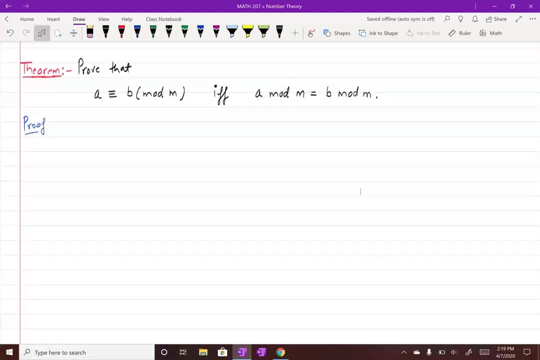 so in our next theorem we want to prove that a is congruent to b modulo m. if, and only if, a mod m is going to be equal to b mod m- since this is a statement connected with an if and only if statement- then you can write the proof of this theorem. 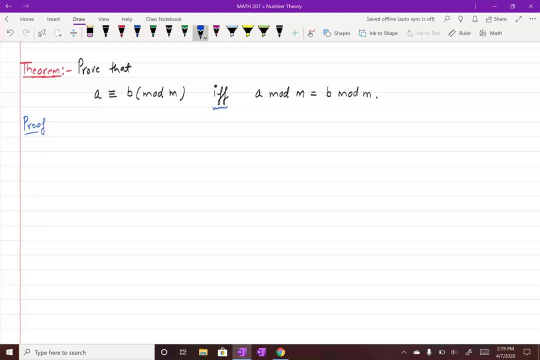 just by first proving that if a is congruent to b modulo m, then this implies a mod m equal to b mod m. and then the second part. you have to prove that if a mod m equal to b mod m, then that implies a is congruent to b modulo m. so in the first part we're going to prove that if a is congruent to b, 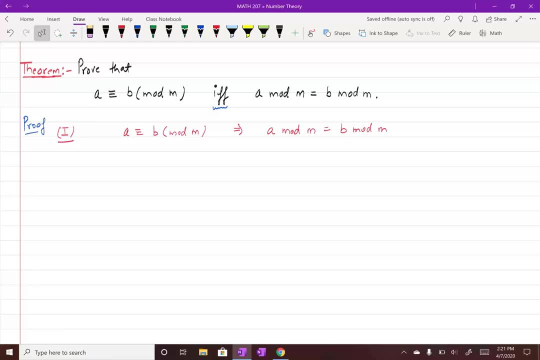 modulo m, then this implies a mod m is going to be equal to b mod m. now to prove this statement we use our diet proof technique, and in our diet proof technique we start by assuming our hypothesis is true. so let's suppose a is congruent to b modulo m is true then, by the definition of: 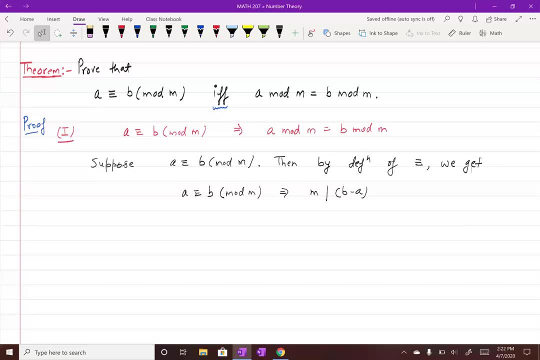 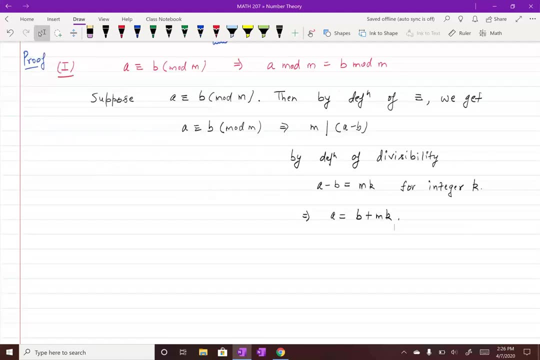 this congruent modulo m, we can say: if a is congruent to b modulo m, then this implies m divides b minus a. so suppose the hypothesis a is coherent to b modulo m is true, then by definition of this congruent modulo m we get that a congruent to b modulo m implies that 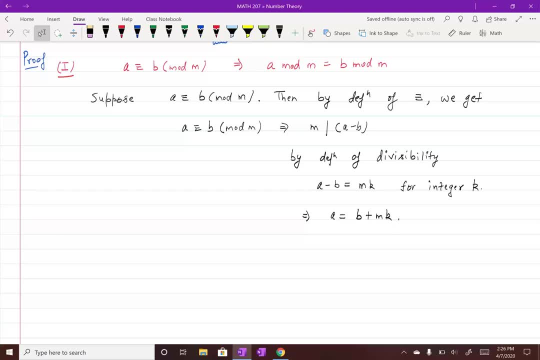 m divides a minus b and then by the definition of a divisibility we can say a minus b can be represented as a multiple of m, for some integer k, where a minus b is written as m times of k and k is an integer. so if you simplify that a can be written as b plus m of k. 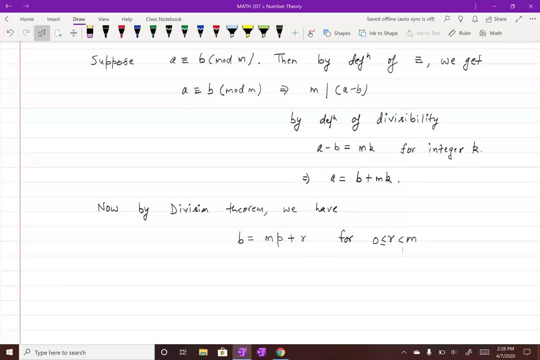 now we can apply our division theorem and we can say: the b integer can be represented as m times of p plus of r. where r is, my remainder is greater than equal to 0 and less than m, and m is my divisor and b is my divided and p is going to be my cosine. 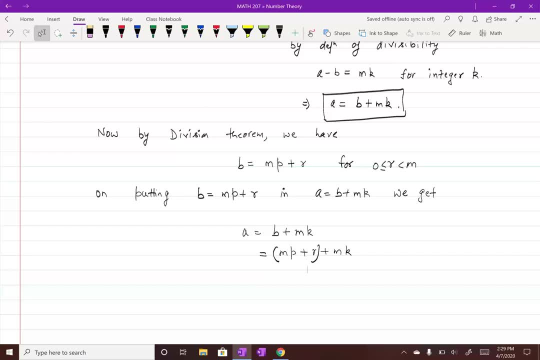 now, if you put b is equal to m p plus r in your a term, which was a, was b plus m of k, so a can be written as m p plus r plus m of k, which you can write as m times p plus k and plus of r. 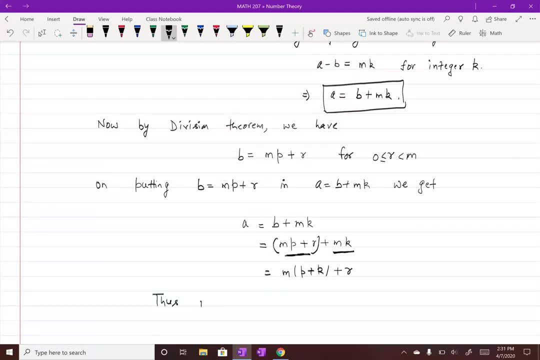 thus we get here that a mod m is going to be equal to r, based on your division algorithm. this is your remainder term, which will be equal to your b mod m, which you obtain from this relation, and r is the remainder term there. so we prove this statement that if a is congruent to b with the modulus m, then this implies: 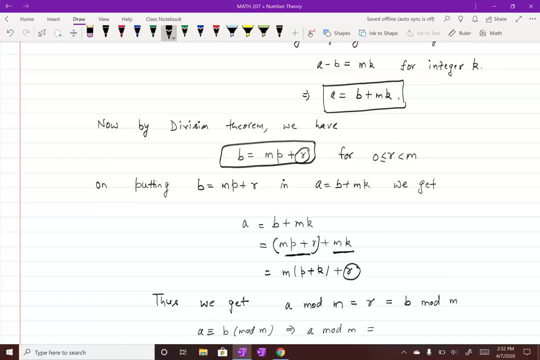 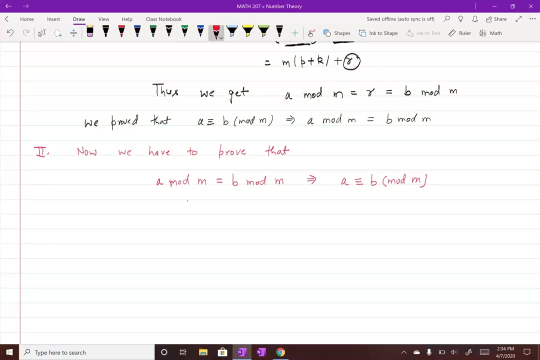 a mod m is going to be equal to b mod of m. okay, so we prove that. okay, so we are done with the first part of this proof. in the second part we have to prove that if a mod m is going to be equal to b mod m, then this implies a is congruent to b modulo m. 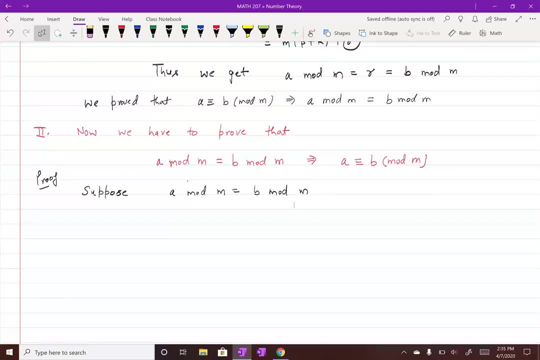 we're going to follow our direct proof technique, where we start by assuming that suppose our hypothesis is true. so that means suppose a mod m is going to be equal to b mod m, and let's suppose we're going to be. both of them are equal to r, where r is greater than, equal to 0 and less than. 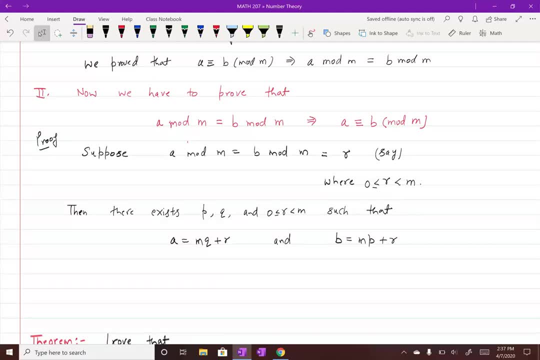 then by the definition of a mod m or b mod m, if that equal to r, we can say there exists integer p and q, such that a can be written as m times of q plus of r And b can be represented as m times of p plus of r. 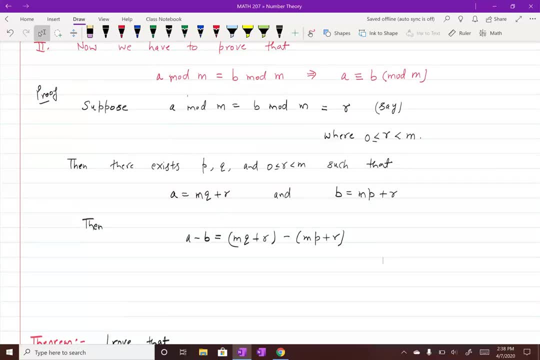 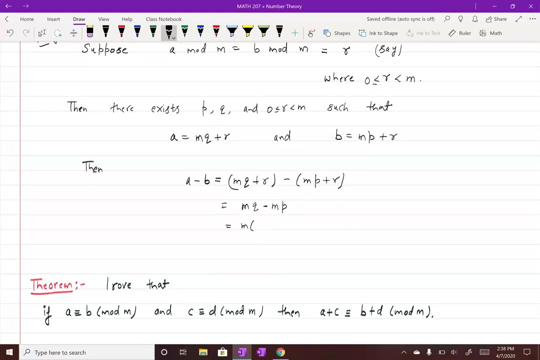 Then a minus p can be written as m times of q plus of r minus m times of p plus of r, which will be equal to m times of q minus m times of p. okay, And equal to m times of q minus p, which you can say, say m times of some integer s, okay. 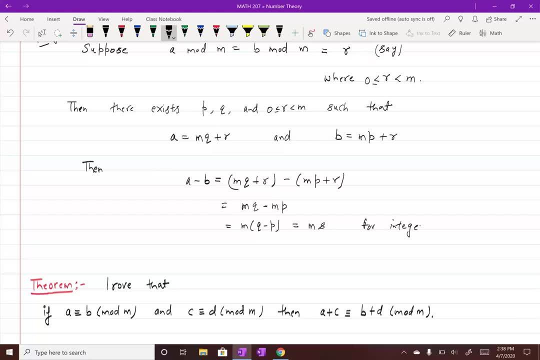 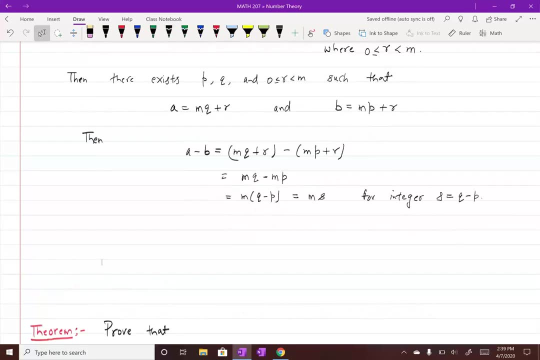 For integer s, which is equal to your q minus p, And since you are able to represent, say, a minus p as some multiple of m, okay, for integer s, then by definition of diffusibility you can say: m divides a minus p, okay. 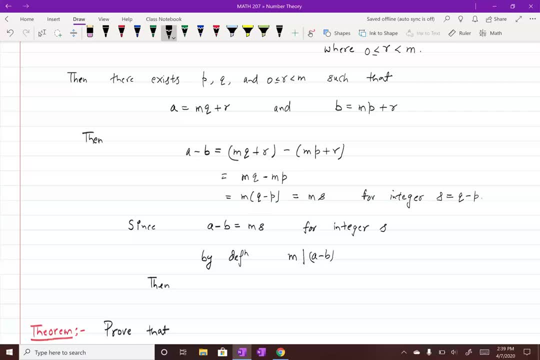 And then by definition say: m divides a minus p is connected with your. a is congruent to b mod m. So we proved that a mod m okay, Equal to b mod m implies a is congruent to b mod of m. 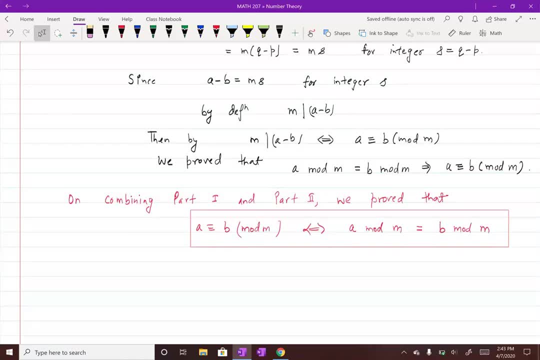 So in combining the part 1 and part 2 of the proofs here, we proved the complete statement And based on that you are saying a is congruent to b mod m if, and only if, a mod m is going to be equal to b mod m. 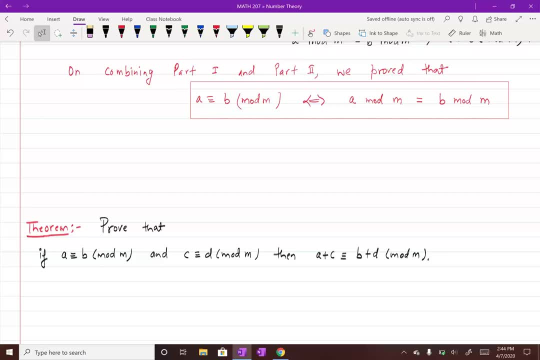 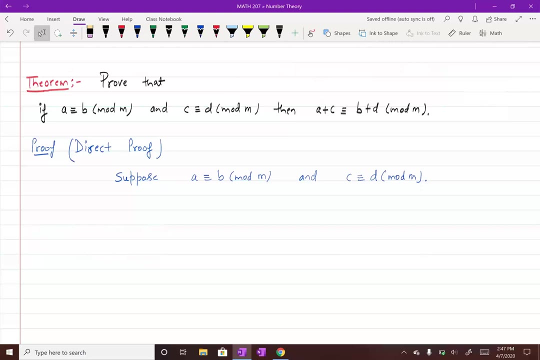 Similarly, you can try to prove this statement that if a is congruent to b mod m and c is congruent to d mod m, then you can also prove that a plus c is congruent to b plus d mod m. So in proving the statement of this theorem, 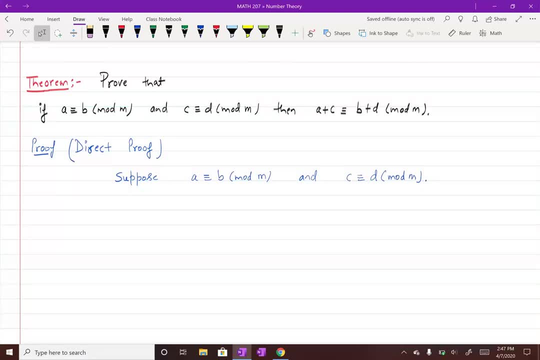 we can use our diet proof technique And based on the diet proof technique, you start by assuming your hypothesis is true. So in this case, suppose a is congruent to b mod m and c is congruent to d mod m. 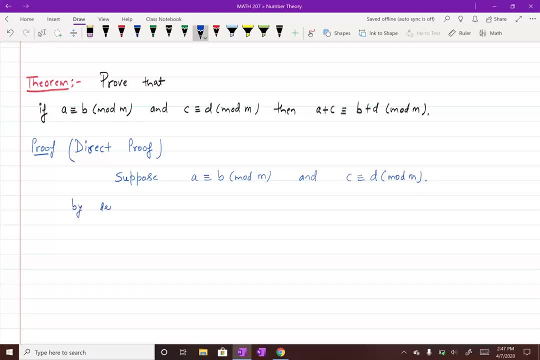 that statement is true. By definition of your congruent, you can say a. congruent to b, mod m implies that m divides your a minus b and c congruent to d. The statement is true. So here we know what c and d are. 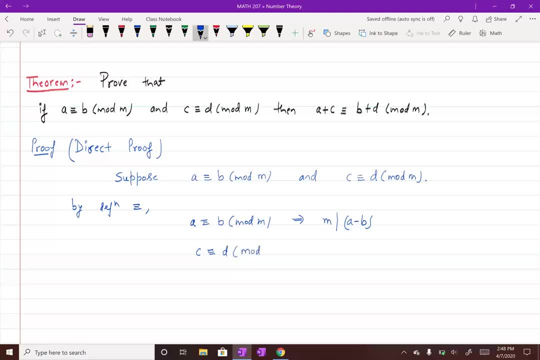 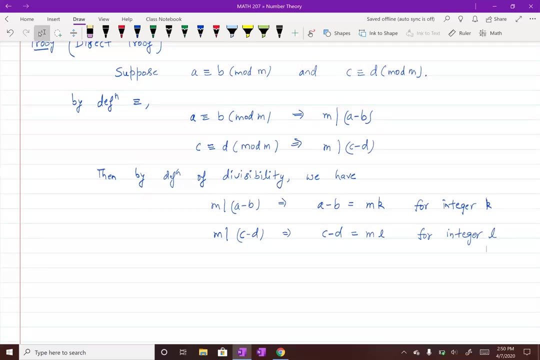 d mod of m implies that m divides c minus d. Then by the definition of a divisibility, m divides a minus b, can give you that a minus b can be written as m times of k, for some integer k and m divides c minus d. that means c minus d can be written as a multiple of. 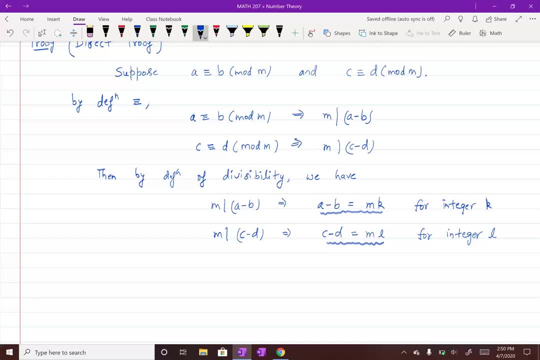 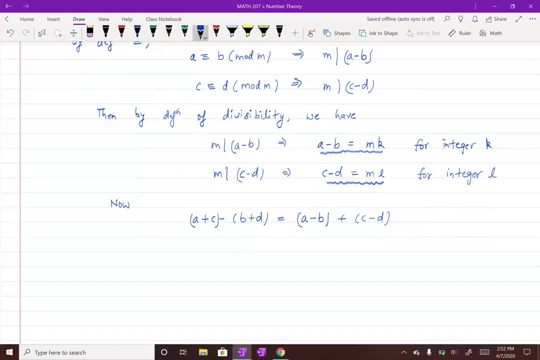 m, which is going to be equal to m times of l. for some integer l, Now a plus c, minus b plus d can be written as a minus b plus c minus d, where a minus b is going to be equal to your m times of k and plus c minus d is going to be equal to m times of l, which can. 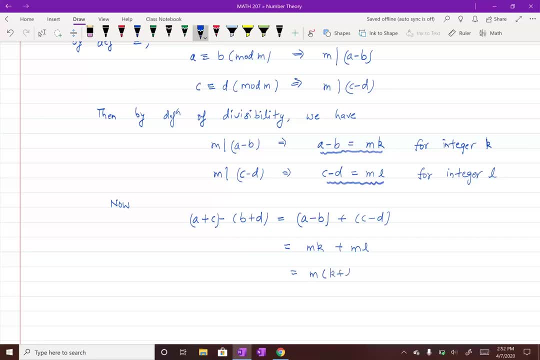 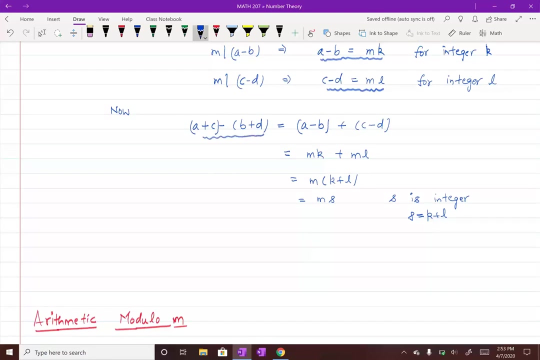 be written as m times of k, M times of k plus l, and can be written as m times of some integer s where s is an integer and s is going to be equal to k plus l. Since a plus c minus b plus d can be written as a multiple of m, so this implies that m 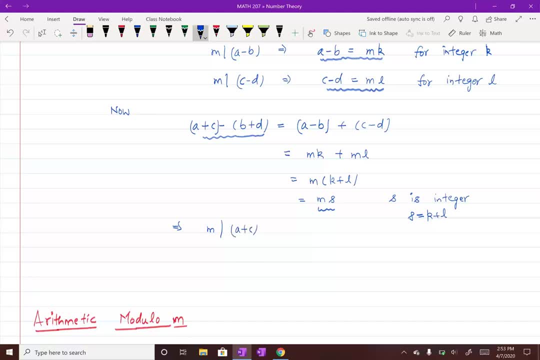 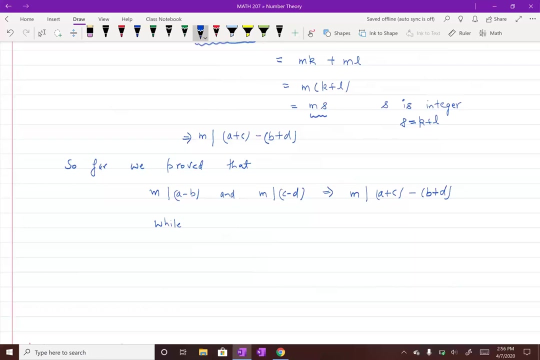 divides a plus c, minus b plus d. Okay, so so far we have proved that m divides a minus b And m divides c minus d implies m divides a plus c minus b plus d, While from our earlier result we know that a is coherent to b mod m if, and only if, m divides a minus b plus. 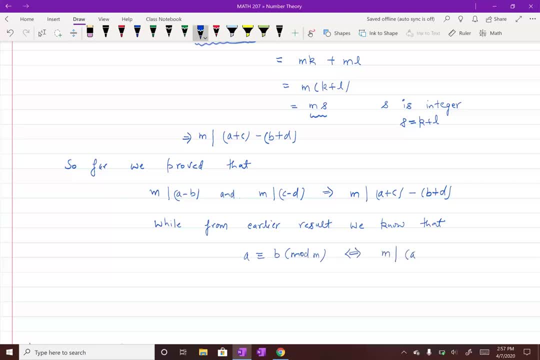 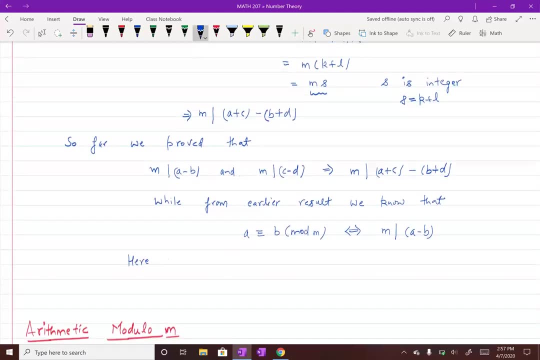 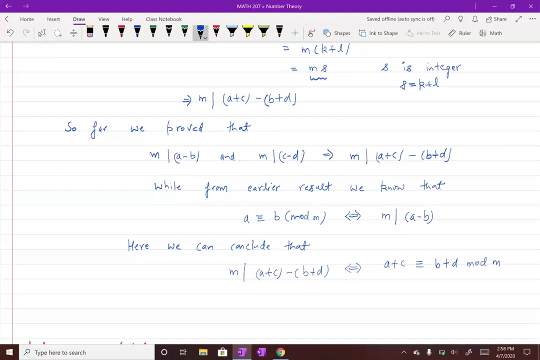 d, P. So here we can conclude that M divides A plus C, minus P plus T, if, and only if, A plus C is congruent to equal to P plus T, modulus M. ok, So on combining, we proved that if A is congruent to B, mod M. 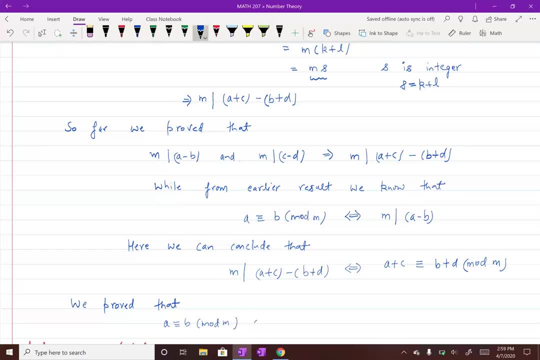 c is congruent to d modulus m, then this implies a plus c is congruent to b plus d modulus m. ok, So this is our final statement, where we proved that if a is congruent to b modulus m and c is congruent to d modulus m, then this implies that a plus c is congruent to b plus.